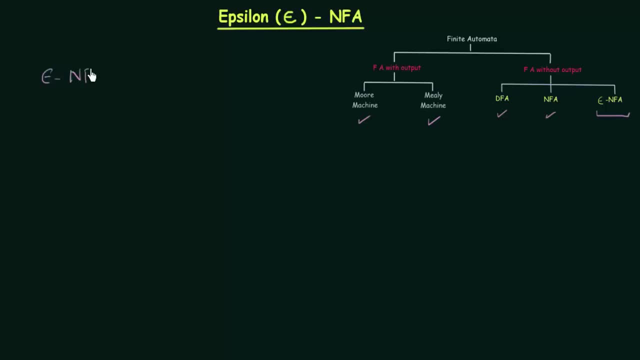 So let's first try to understand. what is this Epsilon NFA. So what is this Epsilon? This symbol right here is called an Epsilon symbol and this Epsilon is used to represent empty symbols, Empty symbols. So it is used to represent empty symbols or non-empty. 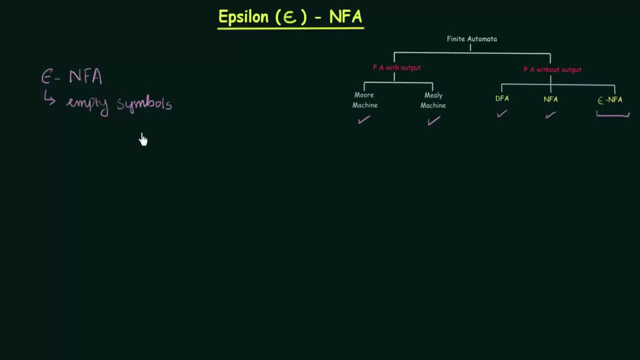 Null symbols, That means it is used to represent nothing. Now that will become clear when we take an example, But before that, let us try to see how do we define this Epsilon NFA. So our regular NFA was defined using five tuples, if you remember, which were Q, Sigma, Q0, Del and F. 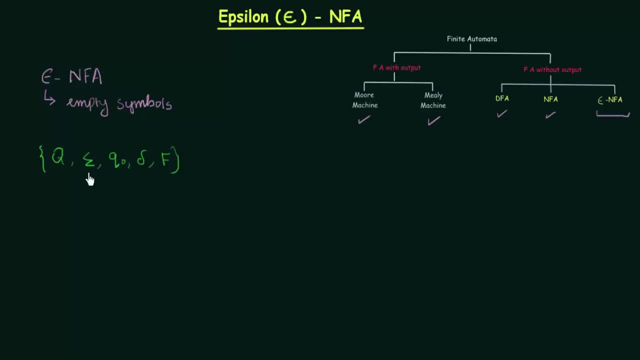 Where Q were the set of states, Sigma were the inputs, Q0 is the initial state, Del is a transition function and F is a set of final states. So even in Epsilon NFA these five tuples are used to define it. 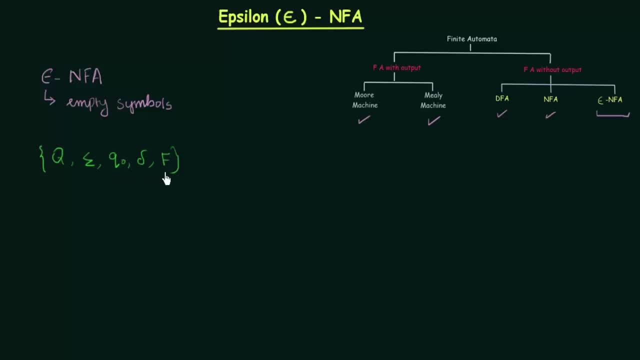 And Q, Sigma, Q0 and F are the same as the regular NFA, And the only thing that is different is this Del. So let's see: how is it different? So in our regular NFA, Del was defined like this: 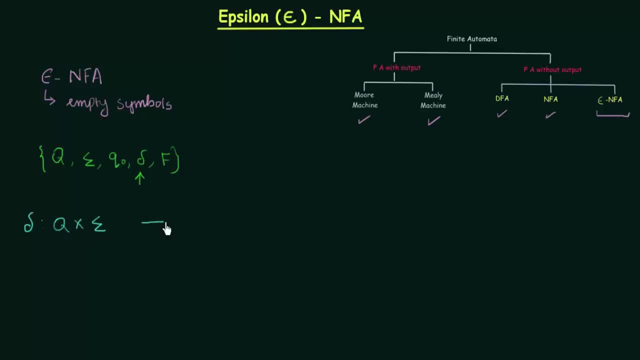 Q cross Sigma To two power Q. So this was the transition function Del. in case of our regular NFA That means any state on getting any input it could go to any of the two power Q states in that NFA. So this was for the regular NFA. but in case of Epsilon NFA what we have is that we have Union Epsilon over here. 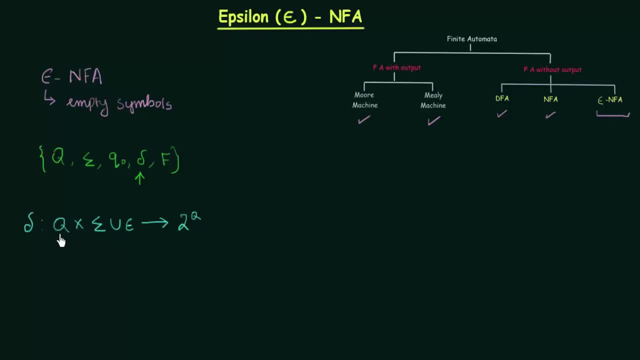 What does this mean? This means that any state on getting a power, a particular input, it could go to any of the two power q states or it could also go to no states and also union epsilon means that the state on seeing nothing or on seeing an empty symbol or 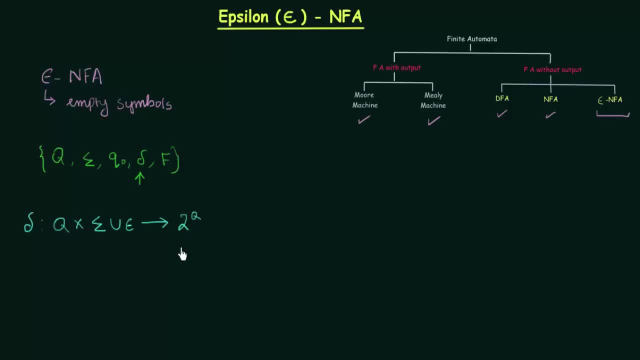 nothing also could go to one of the states. So this will become clear when we take the example. So let me draw an epsilon: NFA over here. Here, A is the starting state and we have another state, B, over here, and let's say we have another state, C and D, here, and D will be my final state and A goes. 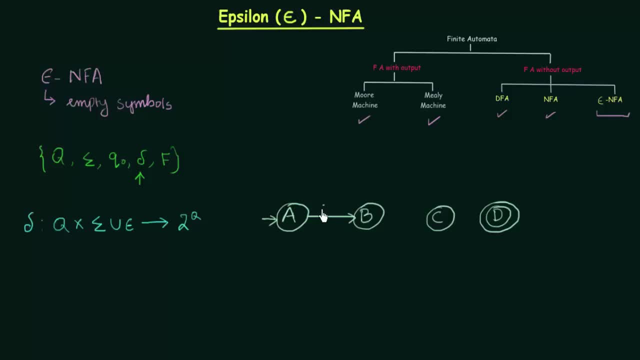 to B on getting input zero and B goes to itself on getting input 1 and B goes to C on getting the input epsilon and C goes to D and it becomes this state, and now we are going to use the yours B forward slash minus zero meter norm. So, since B has 0 input, my final- and D has 0 input. Okay, and now let's look at the etcetera. let's dial C and D and it's 0 for the second one. B goes to C and D goes to negative 1 and D goes to negative 1.. 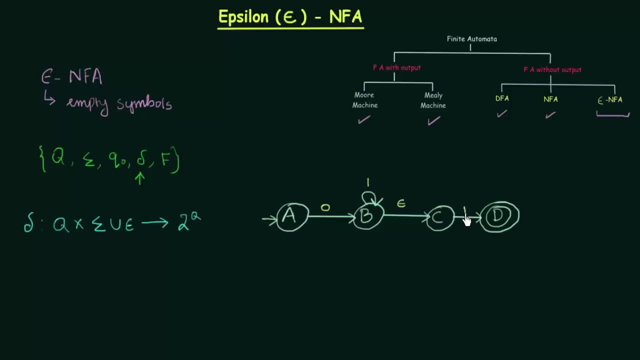 So this is c, 2 and 3 times, 3 times a, prime times b, on getting the input 1 and on getting input 0, C stays in itself. Alright, so this is an epsilon NFA. And how do you recognize it is an epsilon NFA? 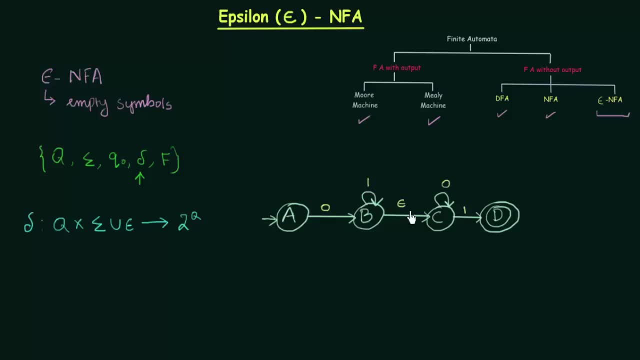 You see that there is an epsilon symbol used here. In a regular NFA this symbol was not allowed. So what does this mean? We have A. A on getting input 0 goes to B And B on getting input 1 stays in B itself. 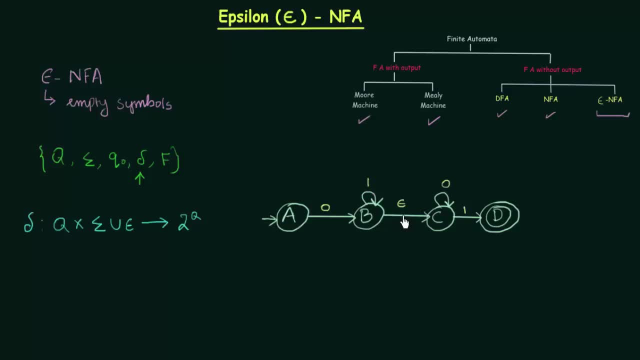 And on getting epsilon. Now, what do I mean by getting epsilon? It means that B on seeing nothing, even on seeing nothing also, it could go to C, And then C on input, 0 goes to C itself and on 1 it goes to D. 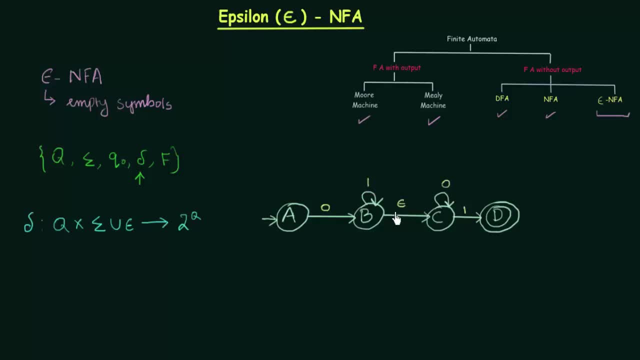 So our main focus is on this epsilon symbol. This means that B- even if it gets nothing, it can go to the next state, C. So that is how the epsilon NFA works, And one thing that you need to remember is that every state on epsilon goes to itself. 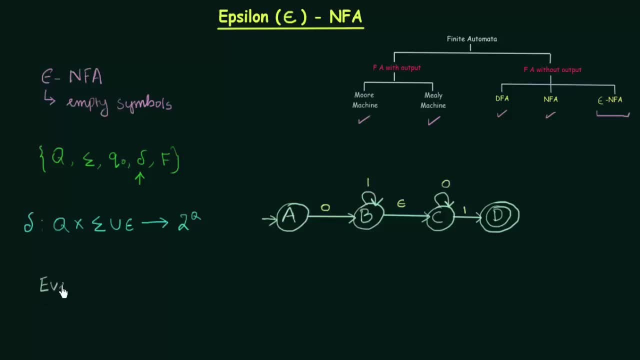 Let me write it down here: Every state on epsilon goes to itself. Now, what do I mean by this? This means that here we have not mentioned any epsilon symbol for this A. But even if it is not mentioned, you should know that A on getting epsilon, it goes to A itself.